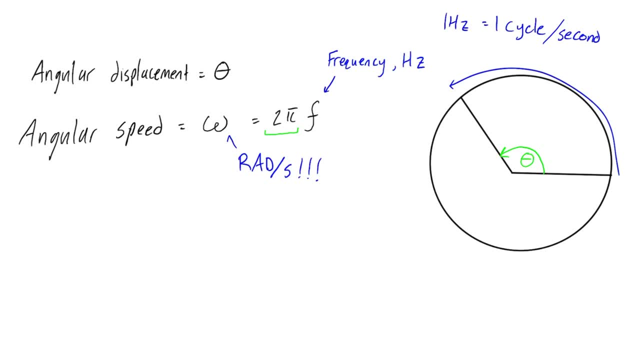 So really, when you look at this expression, you see this: two pi in here all that's doing is converting from cycles- Cycles per second- into radians per second, Because if we have, say, one revolution and we want to convert that to radians, we would apply our factor of one revolution per. 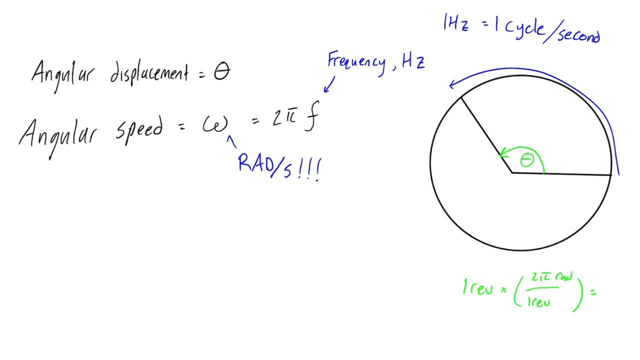 two pi radians And that would give us, basically, those would cancel out and we would be left with two pi radians. So that's all that's going on here is this converts frequency from hertz into radians, So you might also hear angular speed referred to as angular frequency, which would be in 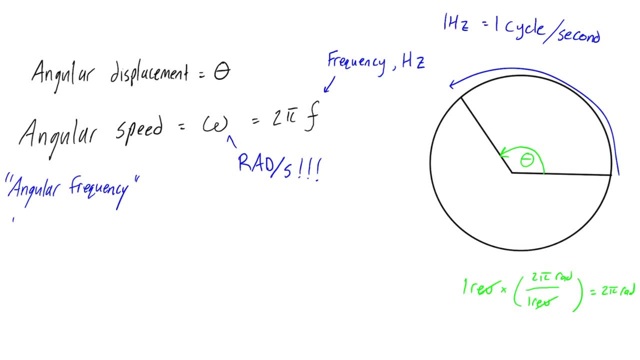 terms of cycles per second, And you also might hear it referred to as angular velocity, And obviously the difference between speed and velocity is velocity is a vector quantity, So we would just indicate the direction, whether counterclockwise or clockwise, And it's the 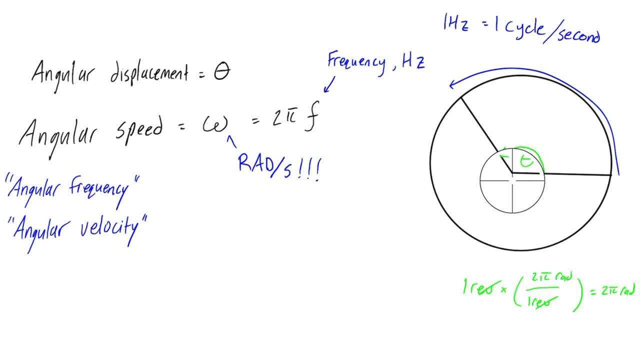 same as statics and moments. You know, basically, use the right hand rule. So you would make your hand and do it, So you would make your hand and do it. So you would make your hand and do it. So you would make your right hand into a fist and put it basically on top of your screen, like 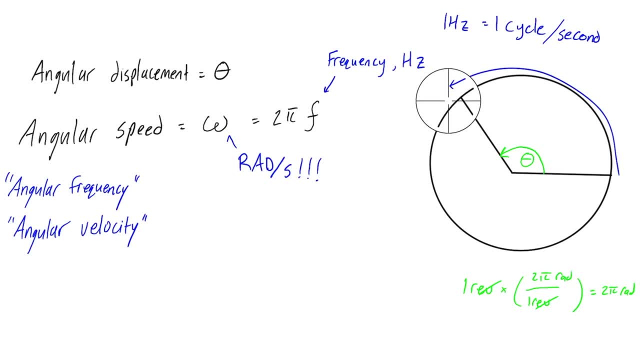 this. Your fingers would be curling around this way, your forefingers and your thumb would be pointing straight out of the screen right here. The coming out of the screen would technically give you your vector direction based on this rotational sense- very similar. 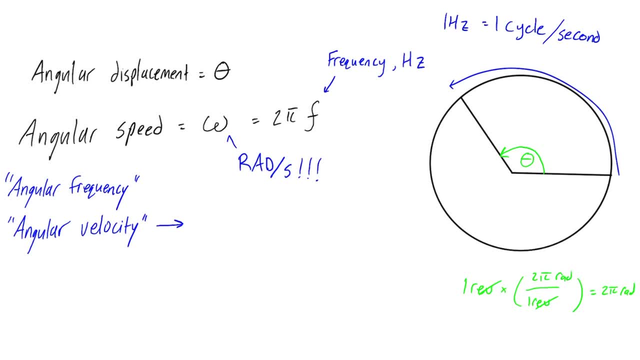 to moments in statics. So just make sure you remember to use the right hand rule if you're dealing with angular velocity- velocity instead of angular speed. but often you can just write the sense, like you can draw that or that, and that's pretty good indication to your professor that you know what's going on. So, anyways, if our angular speed is changing, basically we can, we can define an average angular speed. So we would have omega average And that is really just equal to you. take the average of the values, the initial plus the final, divided by two.